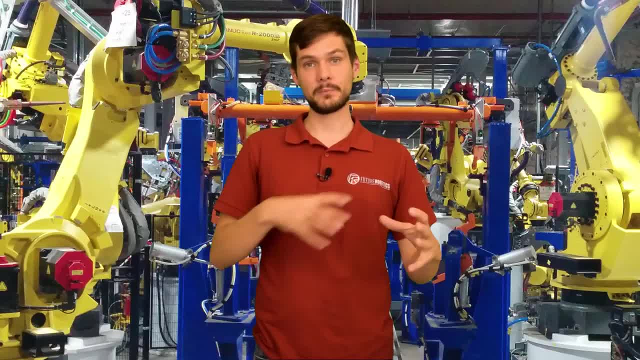 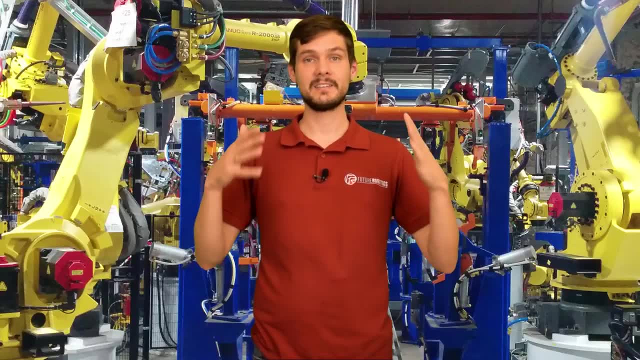 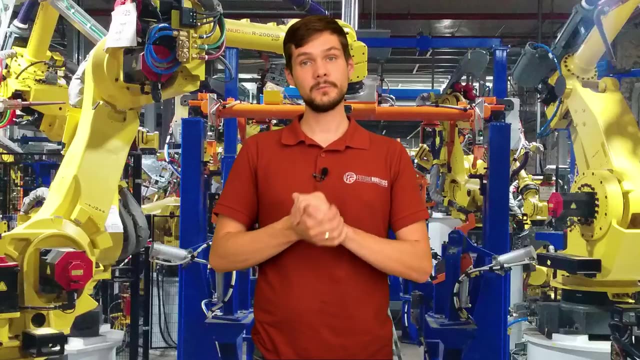 you can see that in the next part. You need to know how to use it so you can actually create the program, jog the robot to the correct positions, and so on and so on. So guys again, go there, take it out and we can jump right into creating the program. So, without further ado, let's. 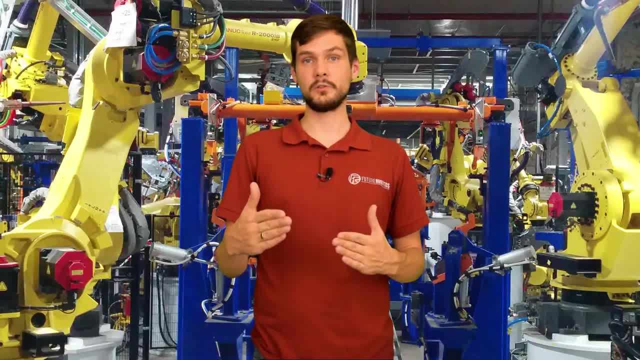 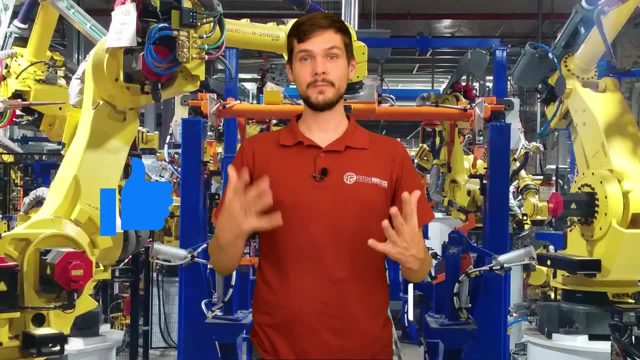 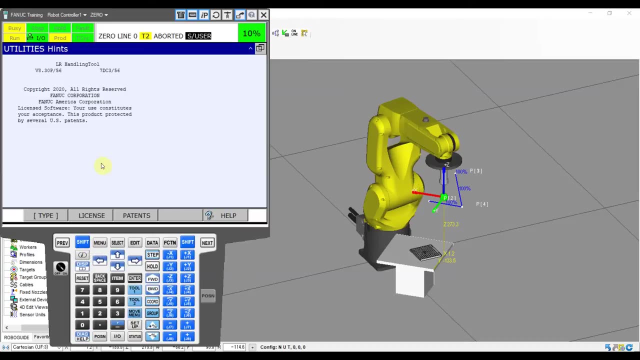 get to the exercises and I'll explain everything to you back there. Oh, please don't forget to subscribe. hit the like button and right now we are ready to go. Okay, guys. so welcome to the exercises. So we're going to create your first. 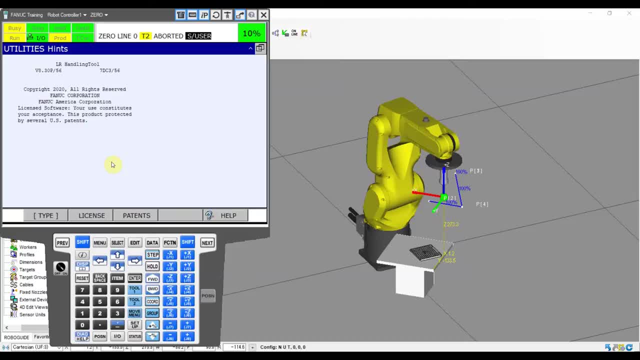 program today and I'm going to tell you a little bit about what type of program we can create. But we're going to focus just on the main program for now. The next one: I will talk a bit more in the next video. Okay, so let's get to it First. 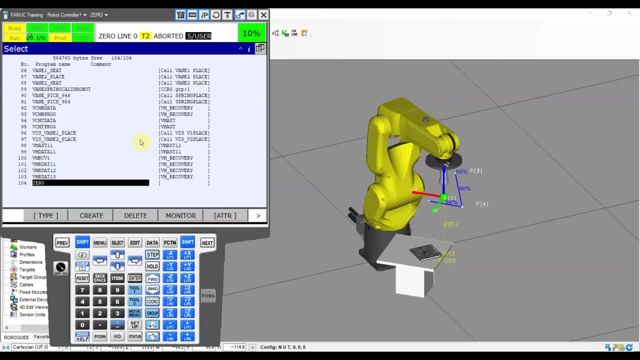 of all, you want to hit select and that's where all of your programs are. Now, as you can see, there is a function menu here. When you hit next, there is a little bit more information. So we talk about that now because you need to know what's going on before you create the program. 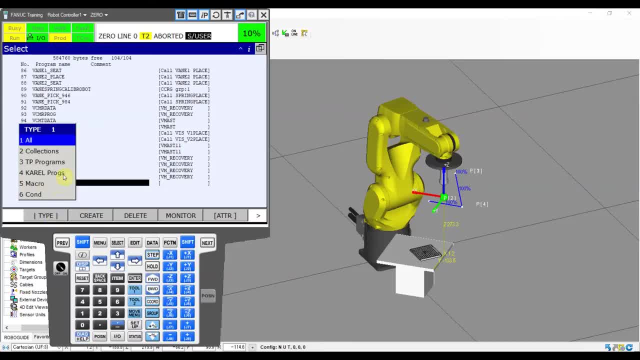 So the first one is a type menu and here you can choose the program type that you want to look at. So, as you can see, we have all programs. You can select collections, you can select teach panel programs, you can select color programs. 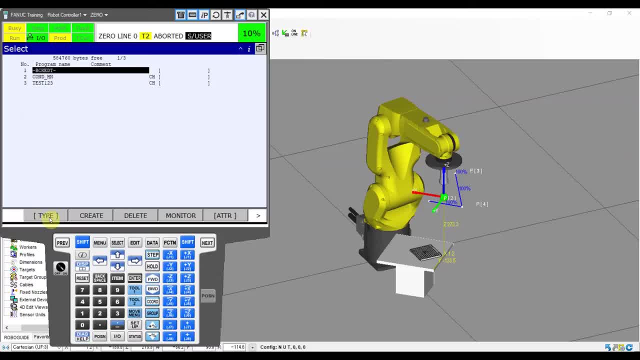 macros and condition handlers, And we're going to talk about all of those in the next videos. Today, we're going to focus on the teach panel programs and that's your main program. In those type of programs, you're going to put all of your 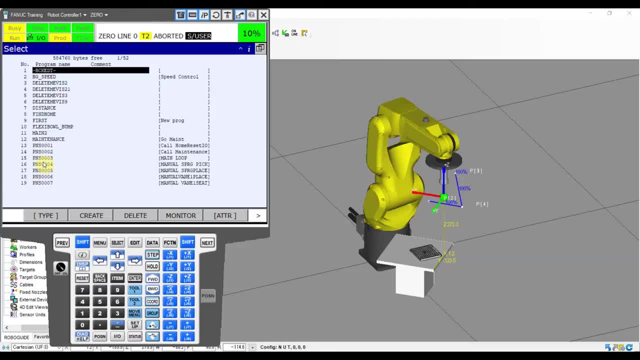 movements, all of your logic. you're going to call sub programs and so on. So we'll start with that one and that's the most common used program. All right, I said we're going to talk a little bit about more about the menus. So the delete one, You can delete the programs with that. 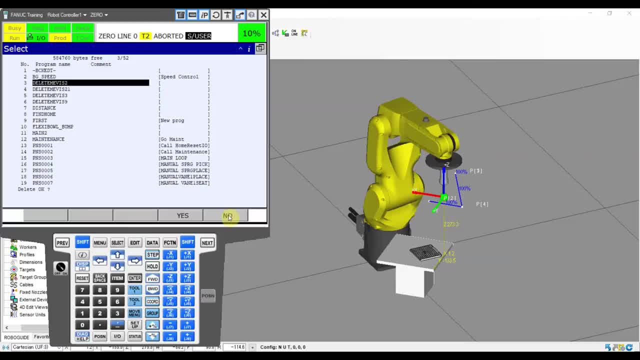 Whenever you hit delete, just in case you make a mistake, you still can say no or yes. When you hit yes, you will delete the program that was highlighted by the bar. The next one is monitor. We cannot use it right now because we are not running any. 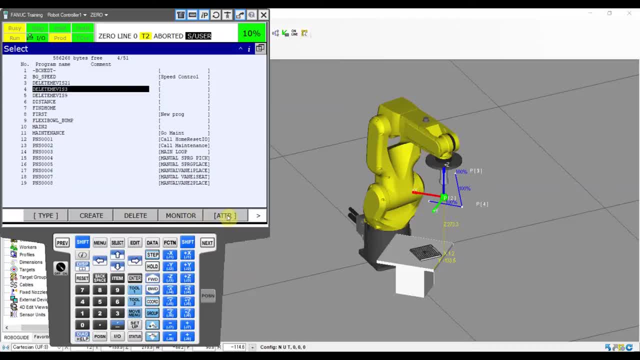 program that's used when you are running a program: Attributes. So attributes are the thing that you can see in here and you can change it. So you can change the comment. So we will show the program comment. You can select protection type. Either it's right, protected, that means you cannot. 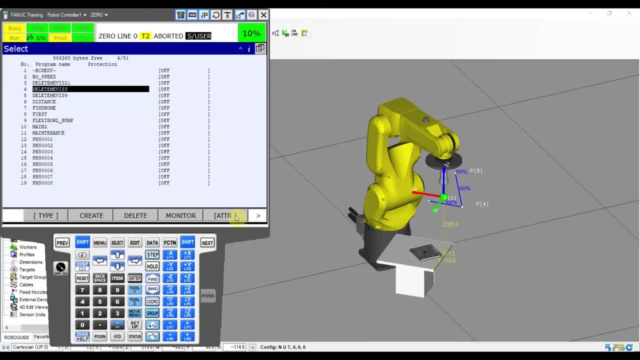 change anything in the file unless you turn off the protection. Last modified. That's very nice, That's very important. So that's showing when the file is. was last opened in editor So you can take a look if someone changed something and if he did when that happens. Really nice option, guys. Remember that one. 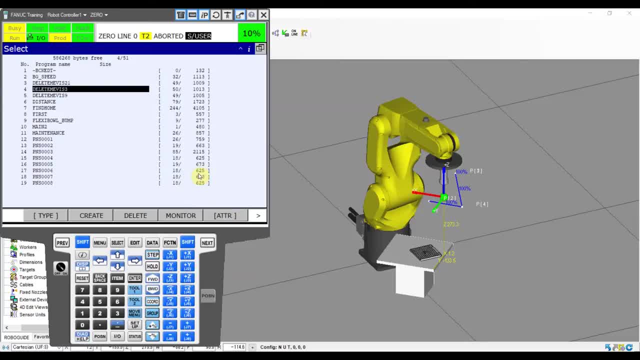 Next one is size, So you can take a look at the size of the file Copy source. So if the program was copied from another program, then you can take a look where it was copied from. So, for example, it looks like the maintenance position was copied from a home program. Next one is the name only, So that will. 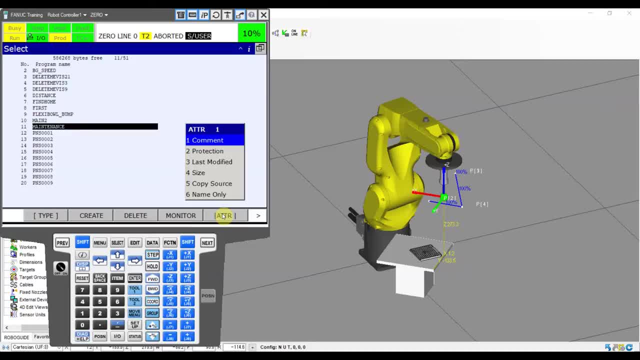 show you just the programs. The one I recommend mostly is probably comment, because you have a program name and then you have a comment that you can take a look at and get a little more information. Okay, In the next menu there are few pretty nice buttons that you want to know. First of them is copy. So 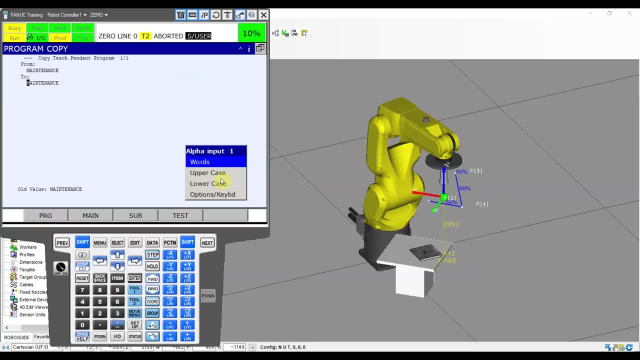 that's what I said. when you copy the maintenance program to, let's say, maintenance one and we hit enter, Do you want to copy? Yeah, we do Right now, when we will change the attributes to copy source, as you can see, our maintenance program is saying that it was copied from the maintenance. Alright, The next. 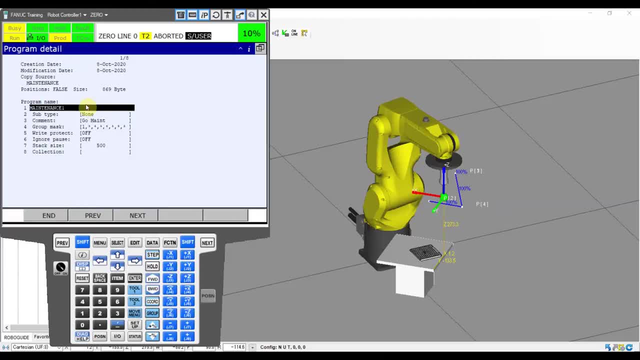 one is detail. So that's showing the program details and we'll talk about those in a moment when we go to a program creation, Because when you create a program you gotta choose all of those Okie dokie. Next one is a load, So we can load a teach panel program. We don't. 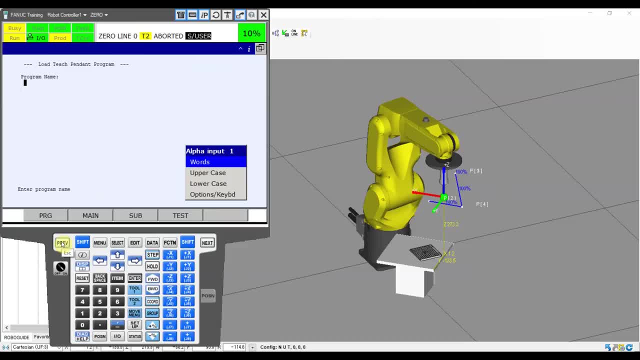 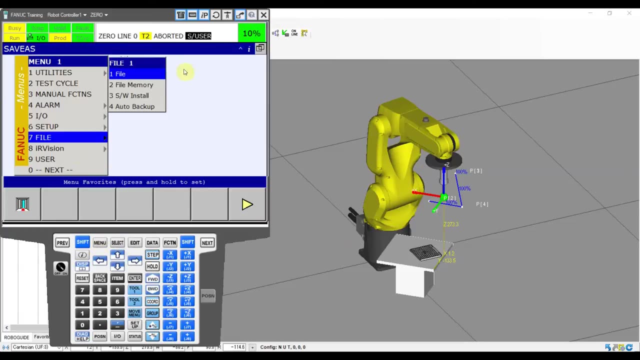 have anything plugged into the USB right now. I will show you in a moment how that works. Next one is save us. So that will allow us to save our program to a directory that we can choose. So let's say we have directory in here, Let's create one. If you don't know what I'm doing, right? 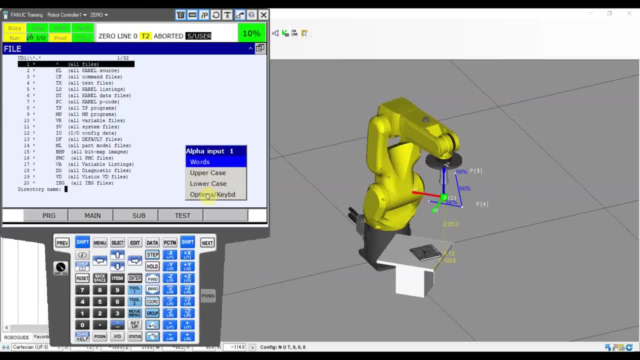 now, guys, you gotta watch my backup video. I'm explaining everything over there: How to create a backup folder and so on. Ok, So when you click save us, we're going to save the file to the directory that I selected before. So when I do do, save, 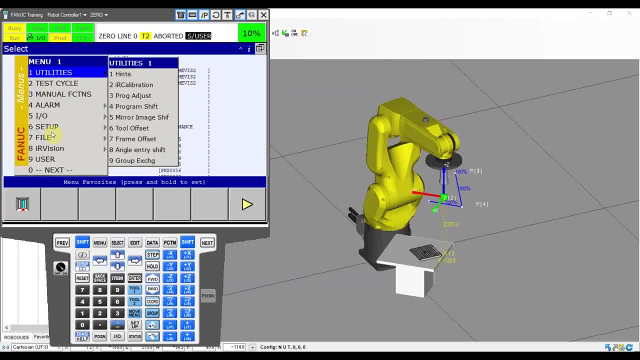 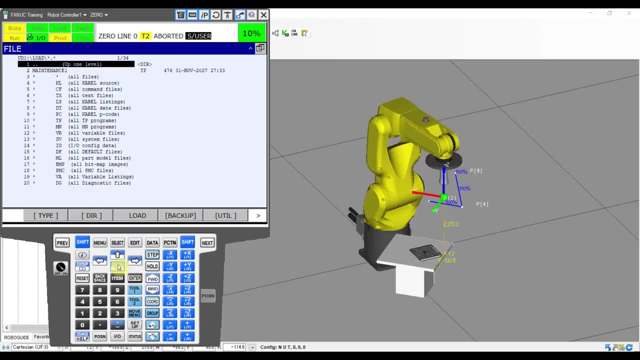 just that one program is copied to that file. That's the directory. I'm sorry. So when we go the UD1 to load, We open it and we have the maintenance program saved as a tp file. Awesome, You can do print, which. 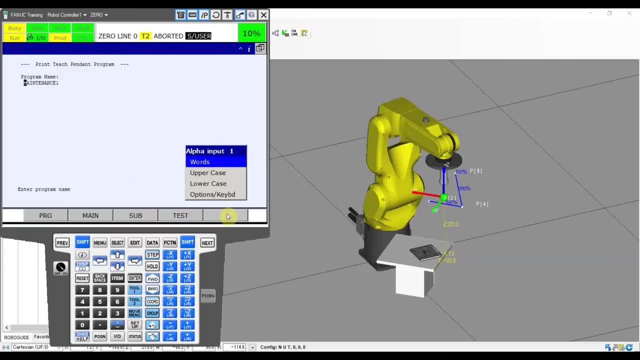 is even more useful. When you do print, remember that you need to pre-select the destination, like I did. So I'm going right now to say to print the maintenance one program to the UD1. And we hit enter, It's going to save it as a ls file. 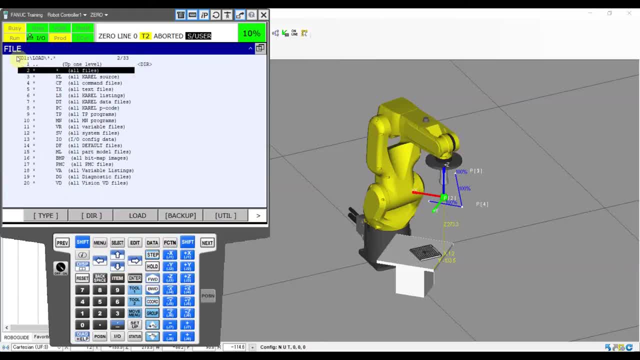 In the destination. So we go again. File UD1.. Load All. See, we have the maintenance one saved as a listening file which can be edited in the notepad, And we have the maintenance file saved as a binary file as a TeachPendant program. Ok, Awesome Now. 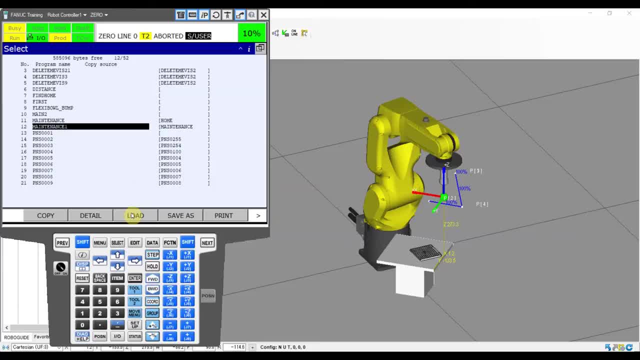 let's go back. Oh yeah, we have the load one left So you can load the TeachPendant, so we can load. But it's saying that already exists and do you want to override Yes or no? So we can override it And it's loading the program out of the 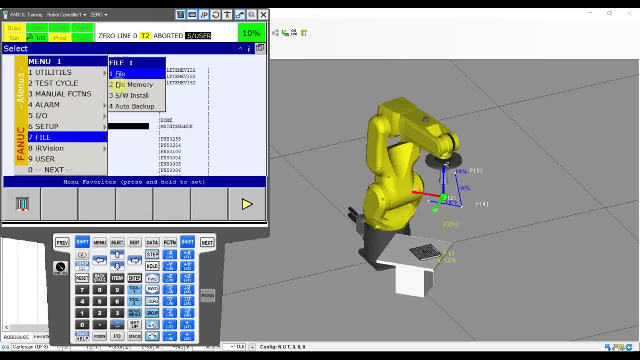 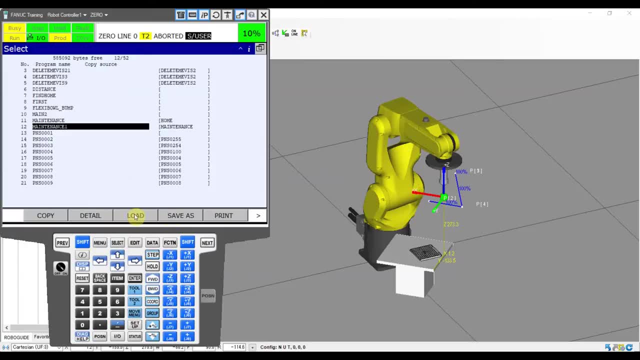 pre-selected directory. So guys would, whenever you select in the file you will try to load from here Whenever you push the load button. I hope that's clear. So let's get to to creating our first program. Okie dokie, So we're going to hit the create button. 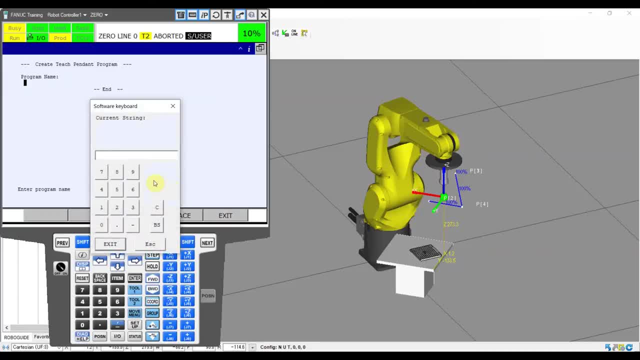 And the first thing you gotta do is you gotta give the program a name. Let's name it first program, First program one. Ok, I hit enter and you're inside the program. Now let's go back, Because I want to show you a few other things. So let's go back. So let's go back to the. 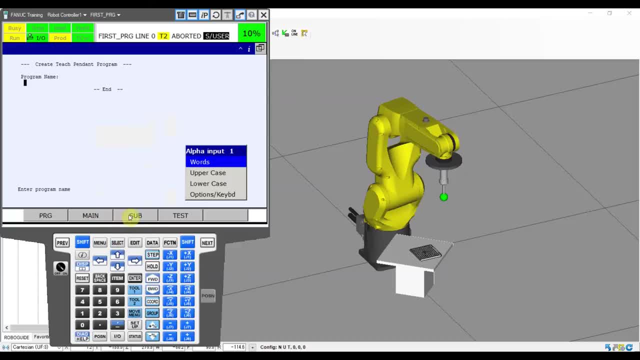 program. So let's go back to the program. So let's go back to the program. So let's go back to the options. So also, when you hit create and you will create, you will give it a name. Oops, Sorry, wrong button guys, One more time. I'm a little bit too used to the 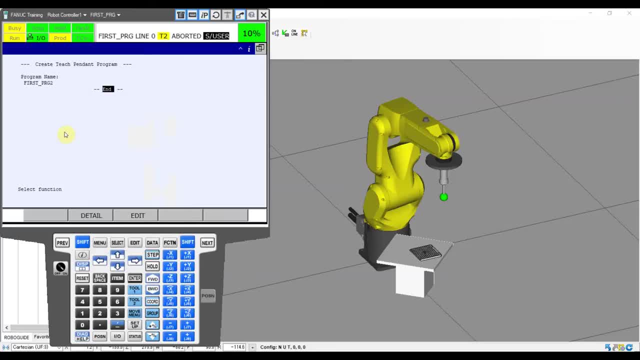 keyboard. Ok, Instead of hitting enter right now, you can hit detail And it's going to take you to the program details that you can edit. When you hit end, you're going back to the program. In case you don't change the program details before you do anything in the program, or actually also after, you can always go to the detail. 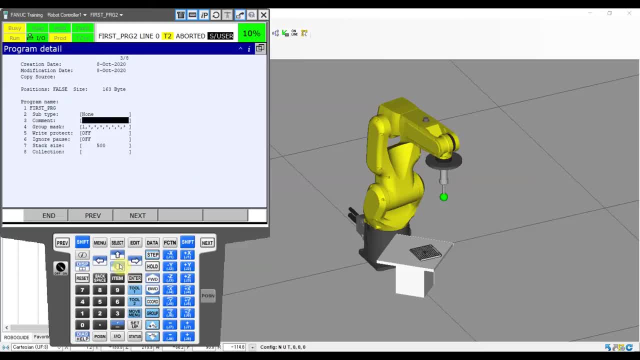 And in here you can change whatever you want. So let's select our program tool that I created. Let's go detail. And right now, what can we change in the detail? The first thing we can change is the program name. So if you want to change the program name, you're going to hit enter And you're going to change the program name to whatever you want. Hit enter, It's changing the program name. 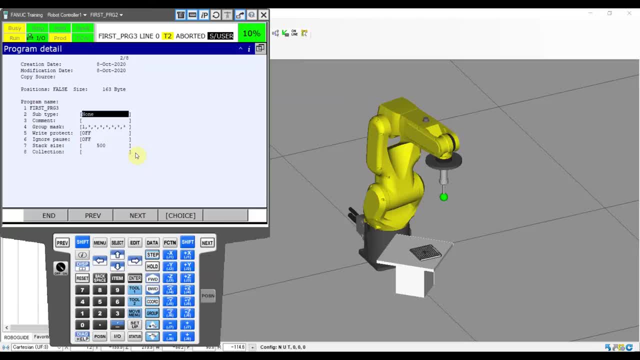 Second thing is subtype, Subtype, And here you're going to select: what type of program do you want to create? Now there are quite a few options. First is- none, None means by default, a teach pendant program with a tp extension, And in the teach pendant program you can pretty much put and do everything. There are no limits, of course, except for the carol logic that can be used only in the carol programs. 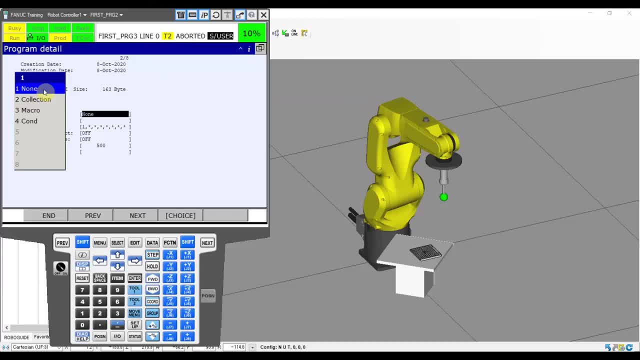 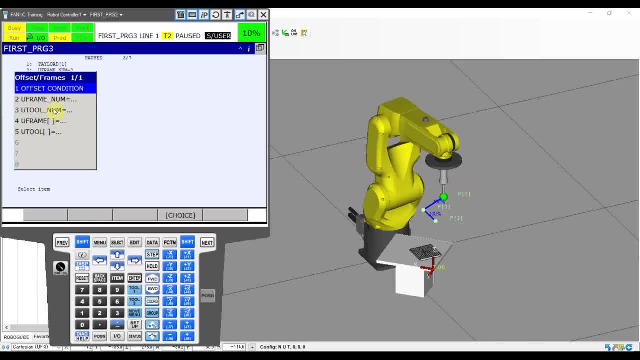 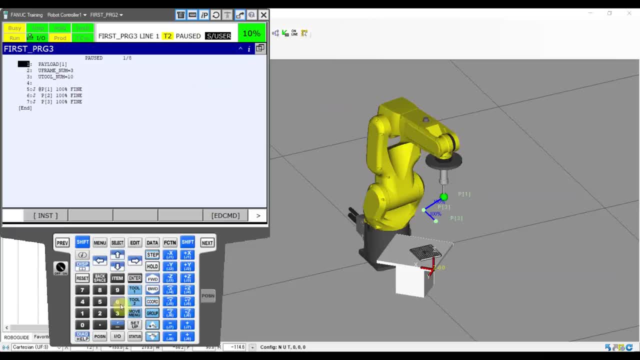 selecting the correct frame and collect tool for the movement. so when you executed we don't have any problems. we're getting overload because the pilot one is not defined. now I want to show you why. because if you will select a wrong user frame and you will try to run the program, it will say that you 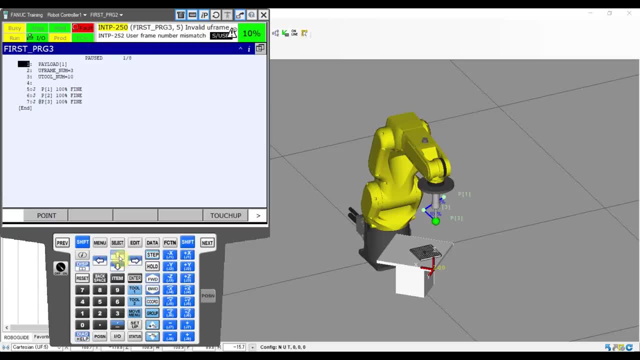 have invalid user frame selected but when you run through the first lines, so if you would not have doubt those defined and you want to run it with those user frames, you're not able to, but as soon as you define them and run shift forward. do you want to start from a different line? yes, we do. the robot is. 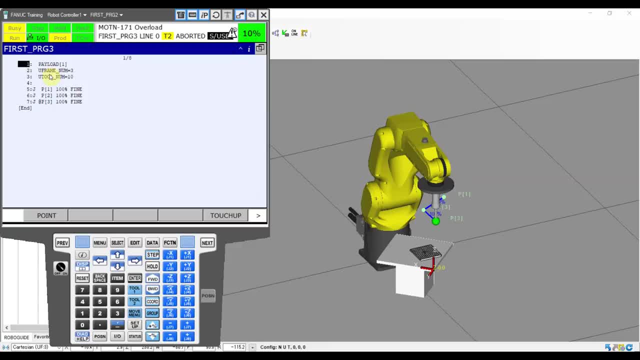 overwriting whatever you had selected with those and you're able to run your whole program. okay, guys, that was a very simple program, but you know how to move the robot right now. you know how to create your first program, you know how to add the points and that's the first. that's the big start for us. so in the